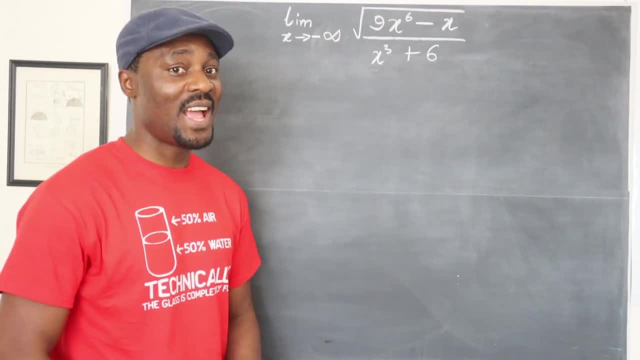 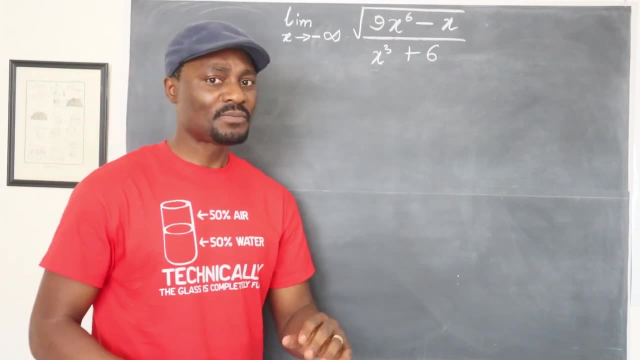 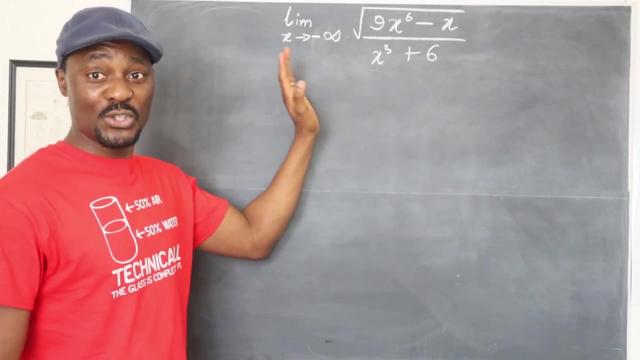 videos. this time, School is starting back up again and we've got to learn, Okay, so let's go into this. The only thing that's going to be new today from my previous videos is the introduction of the negative sign, And I'm just going to answer the question from the beginning. So if you know, 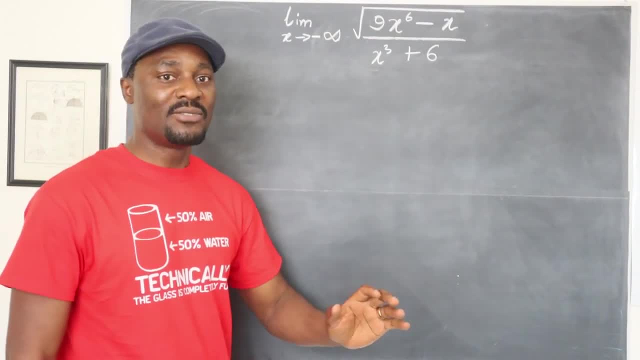 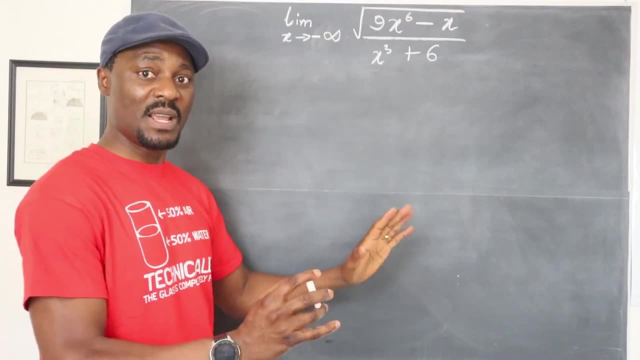 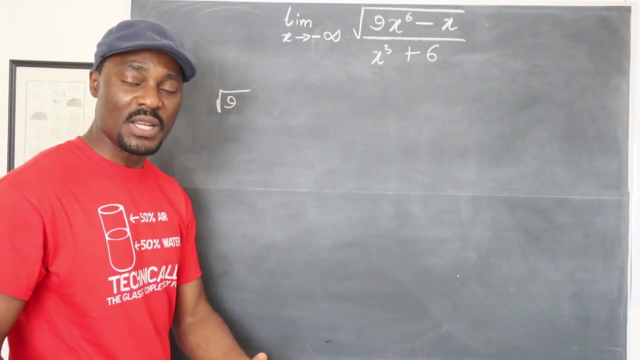 what to do with the rest of it. just go ahead and stop watching. Okay, because this negative sign is going to be important. when you take the square root of a number- And let me explain that to you. So let's say you take the square root of nine, The natural thing for you to gravitate toward 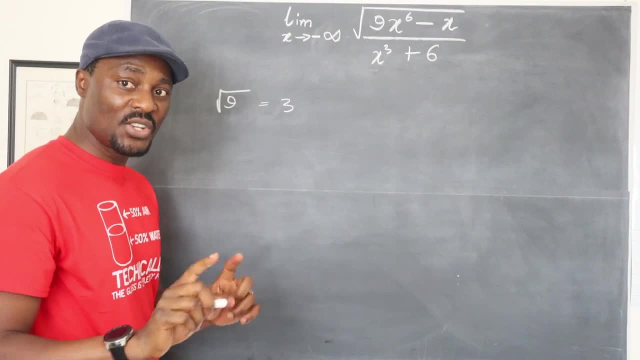 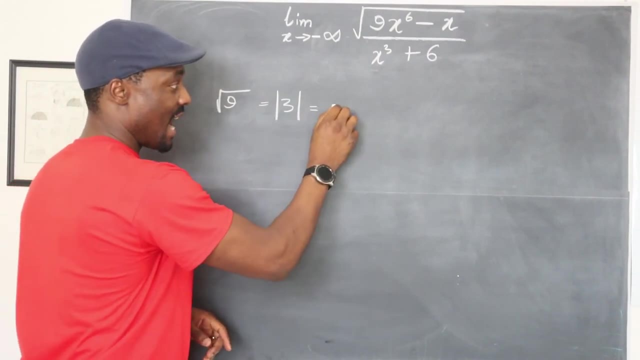 is that the answer is negative. So let's say you take the square root of nine, The answer is three. But let's not forget that the square root of nine is the absolute value of three, which means it is either positive three or negative three. It's either of these two. 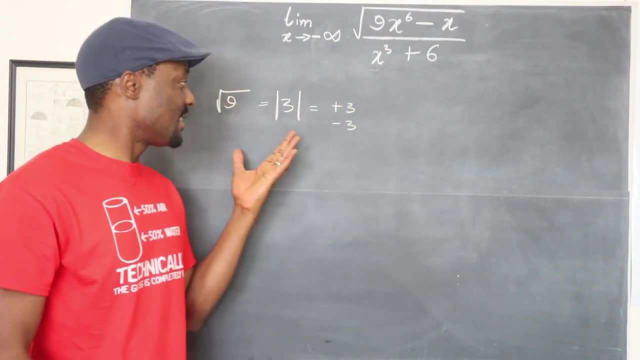 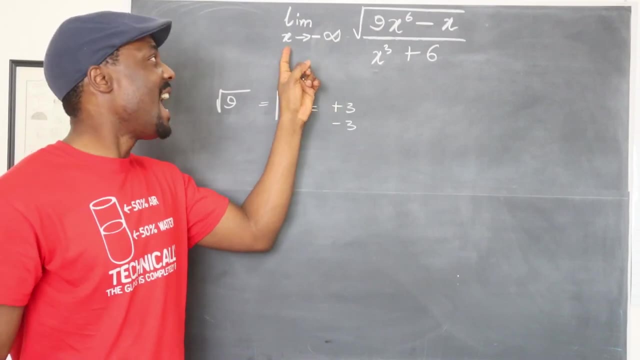 depending on the situation you're in. So, in this case, how do we know if we're going to go positive or negative? Well, it actually tells us, okay, that x is approaching negative infinity. So x is a very negative number, Okay. 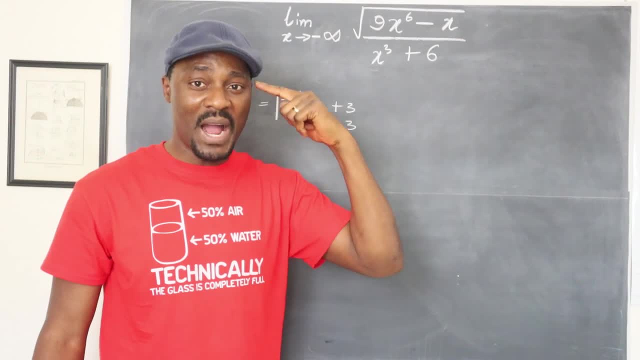 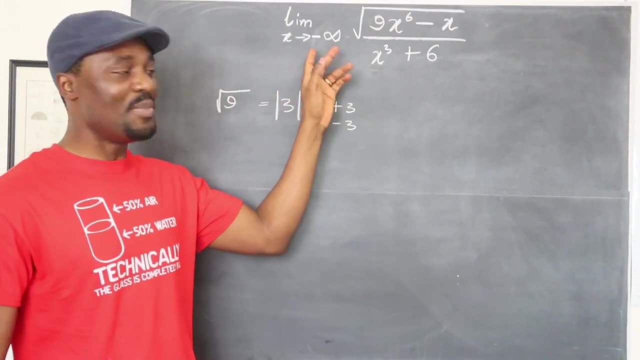 so by the time you take the square roots of what's in here, your mind should tell you that it's going to be negative. You won't take the positive option, you'll take the negative option. That's the only thing you need to note here. Well, the rest of it is up to you. But if you want to see, 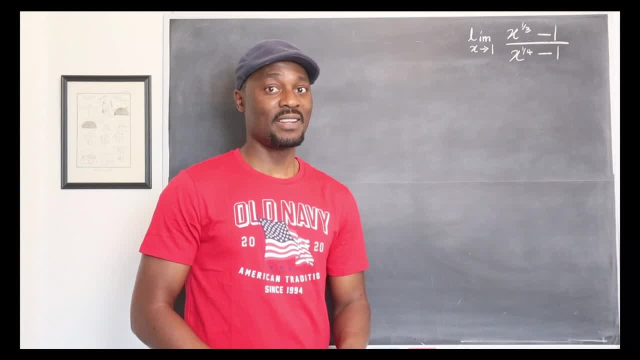 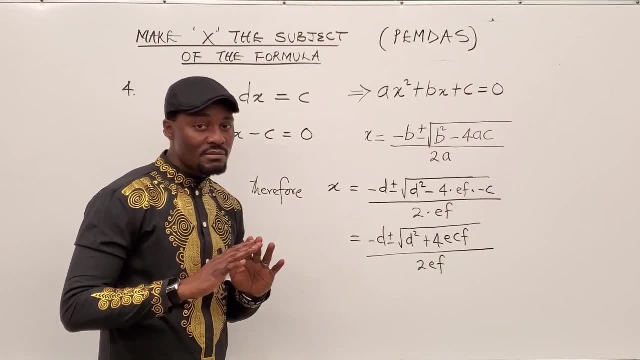 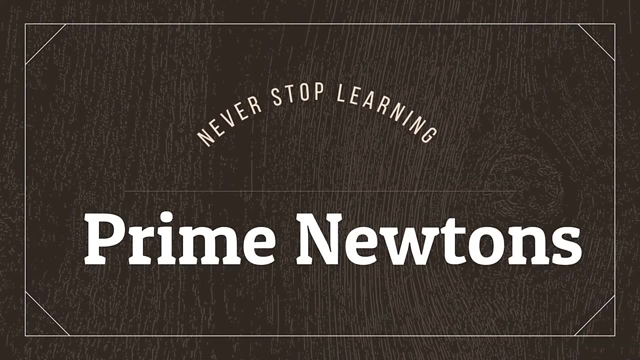 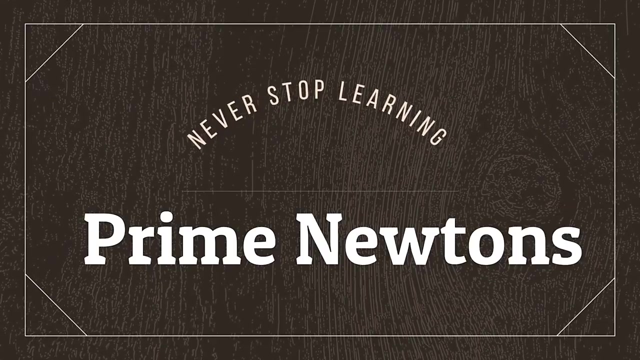 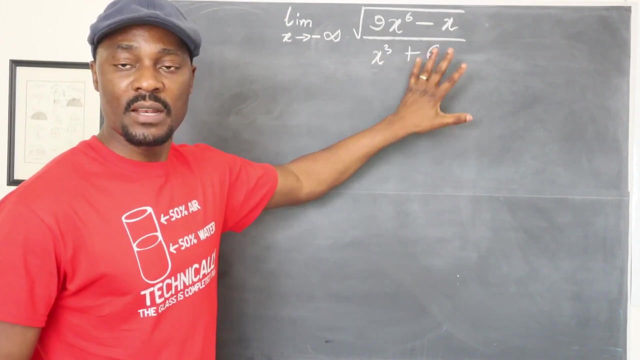 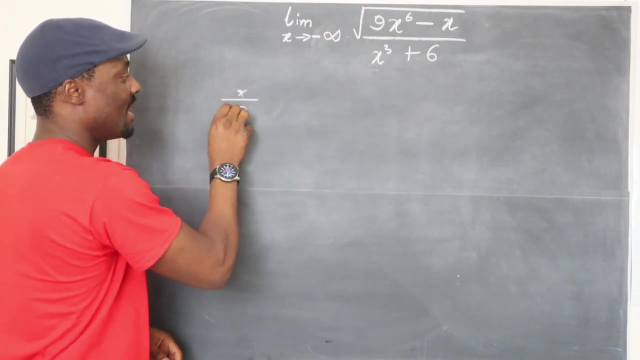 how I do this. why don't you stay with me? Okay, the first thing you would do is to create rational terms in the problem you're trying to solve, because you want to introduce infinity so that you can get something divided by infinity. so your answer will be zero. Okay, you don't want to have zero under and zero. 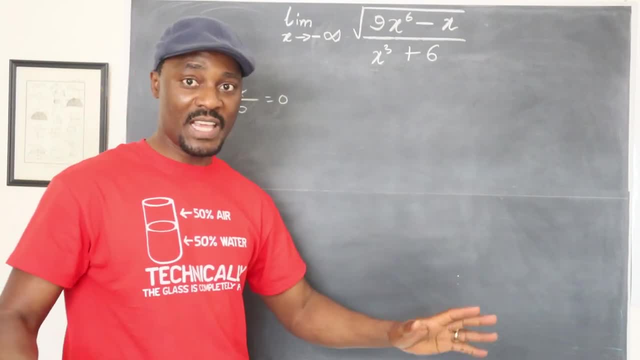 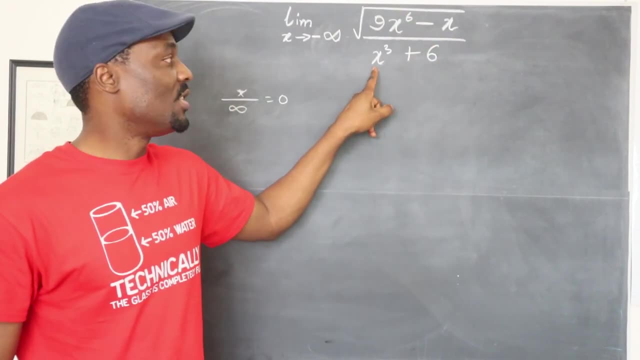 on top, because if you do that right now, that's what you're going to get. But we don't want to get that. What you want to do is to divide this by something, and your best choice is the highest denominator. Okay, the denominator with the highest exponent is what you want to do, So let's. 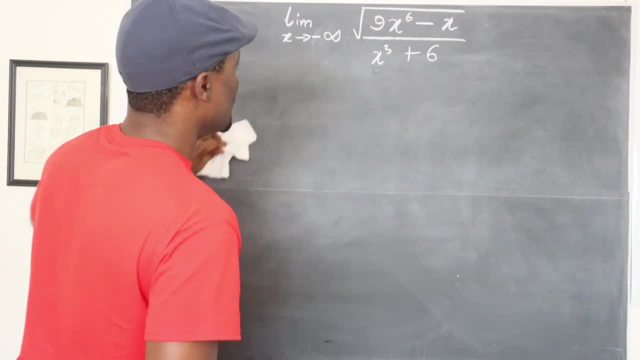 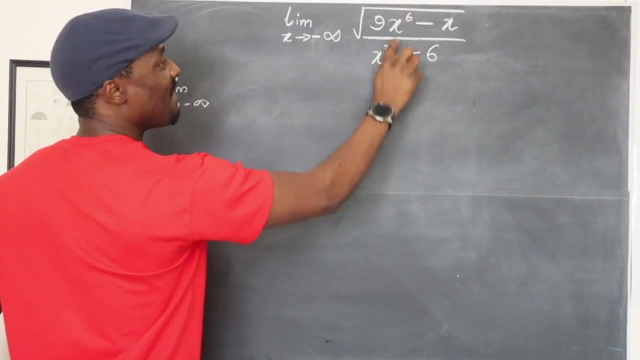 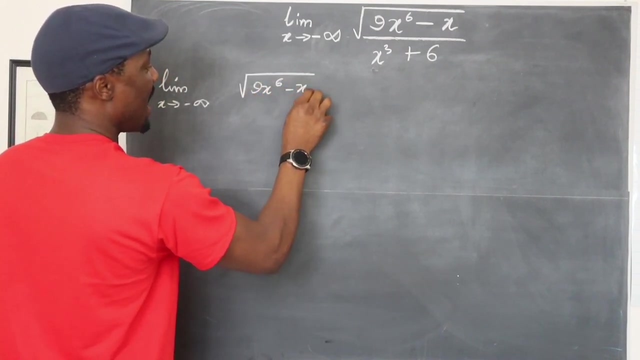 do that. So I'm going to write this as the limit as x approaches negative infinity, I'm going to divide everything by this, So, which is going to be the square root of 9x to the 6th minus x, divided by x cubed, divided by x cubed, plus 6 divided by x cubed. So 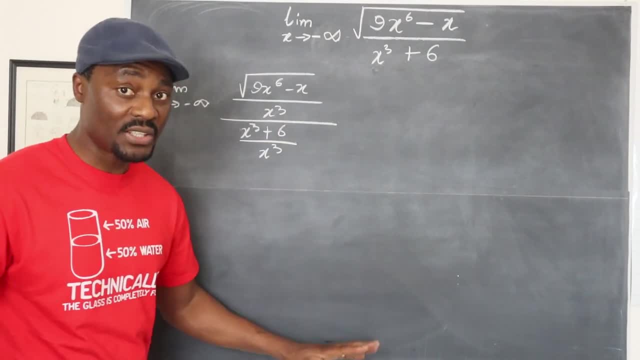 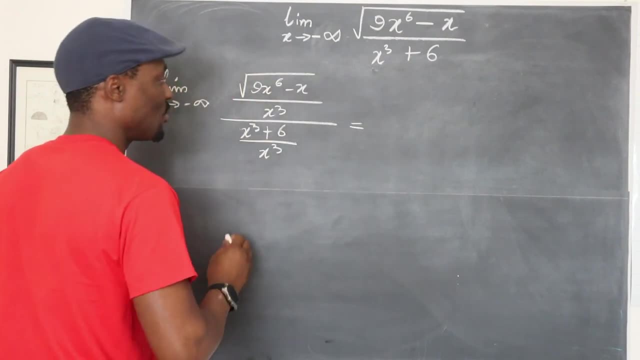 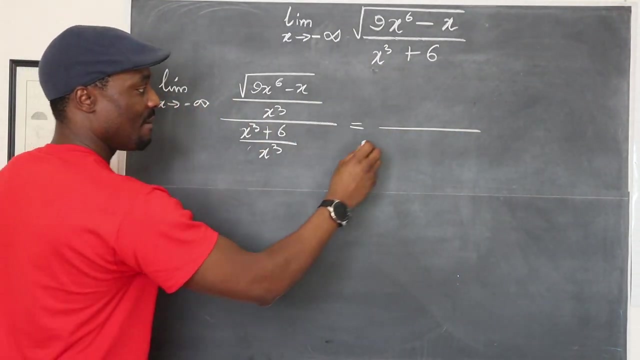 because I divided both top and bottom by the same thing. I have not changed the question, But now I have given myself a way out of this situation. So at this point you can break up this. the denominator You can break this down, You can break this down. You can break this down, You can. 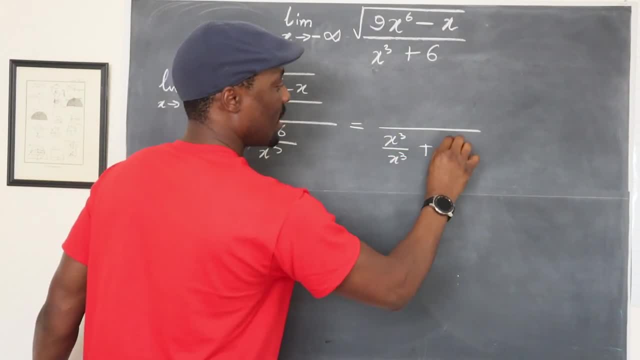 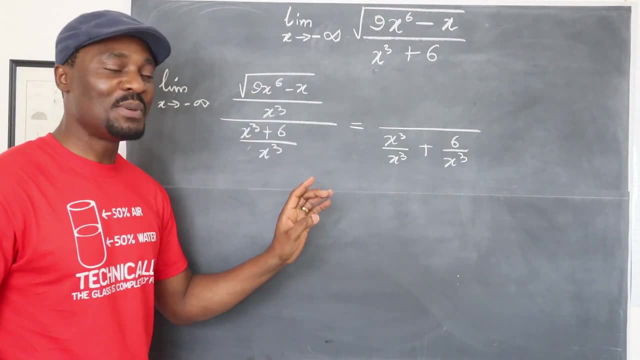 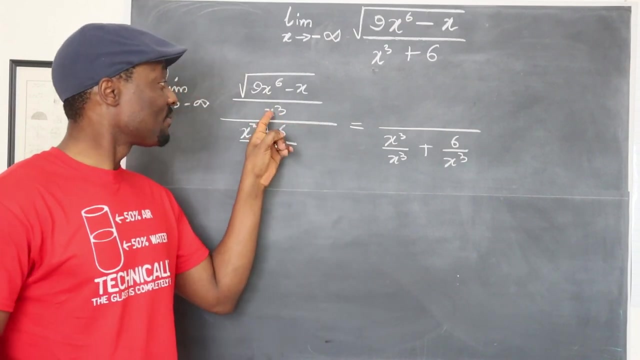 break this up into x cubed over x cubed plus 6 over x cubed. Okay, that's allowed in algebra, But you cannot break this up like this, because these two are bound together by the square root side. So for you to break these two up, you have to sneak this x cubed under the square root side. 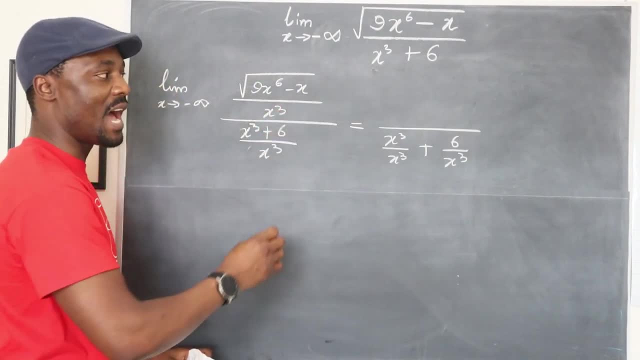 and that makes it possible for you to do. And how do you do that? Let me show you what you have to look at. Look at this: So you have to break this up. So you have to break this up, So you have to. 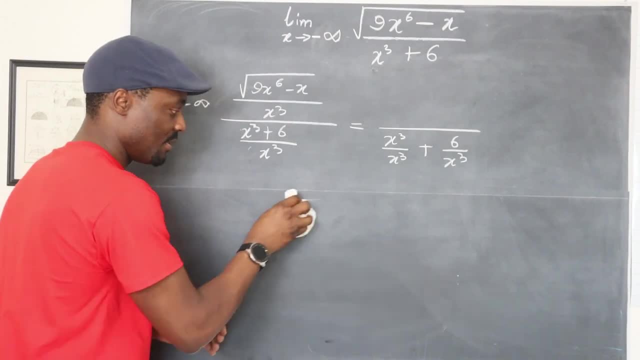 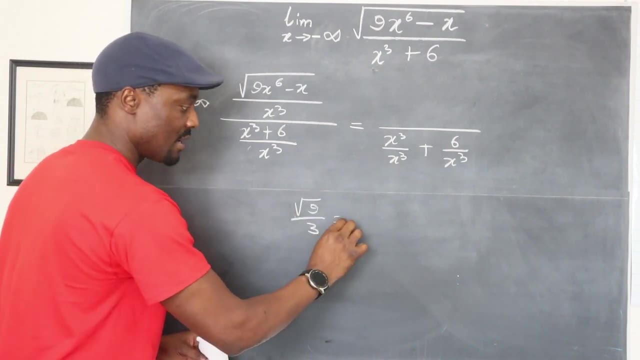 look at this expression: Square root of 3,. let's make it square root of 9 so we can get an answer. So square root of 9 divided by 3.. Well, we know our answer is going to be plus or minus 3.. Okay. 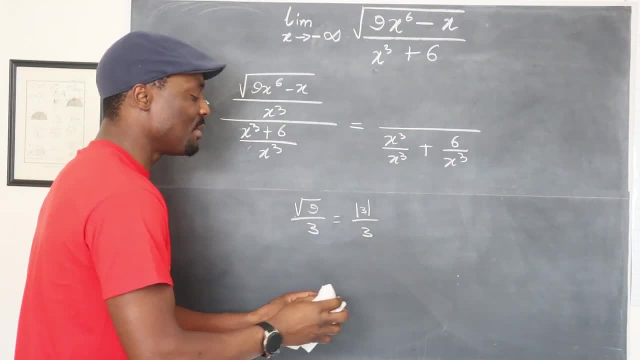 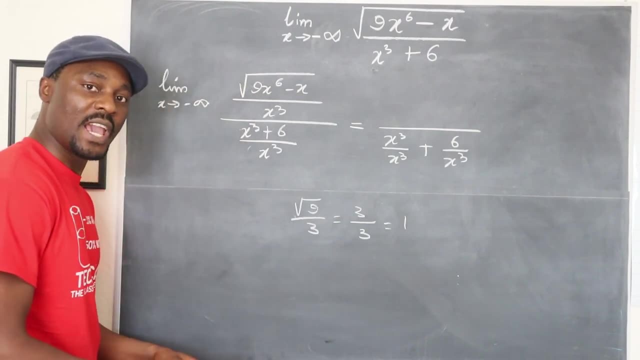 I'm just going to write absolute value of 3 divided by 3.. Let me just write what everybody gets. Okay, I'm just going to write 3 over 3.. Your answer is 1. Okay, but instead of me. 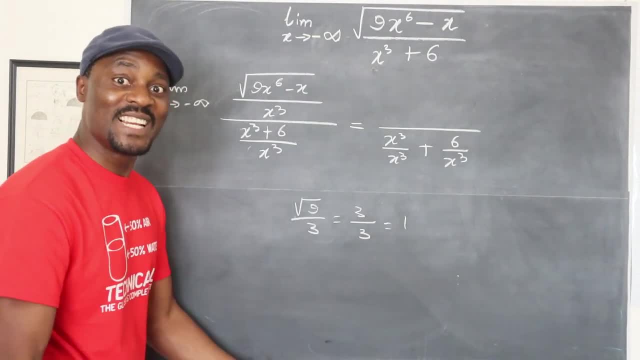 this is easy, because I know this is easy. I know this is easy. I know this is easy. I know this is square root of 9.. What if I didn't know the square root of 9?? Oh, I didn't know the square root of. 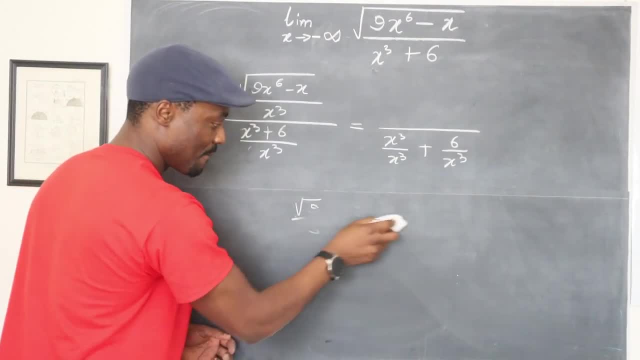 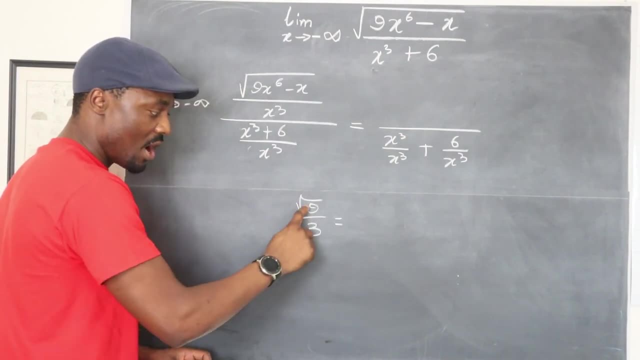 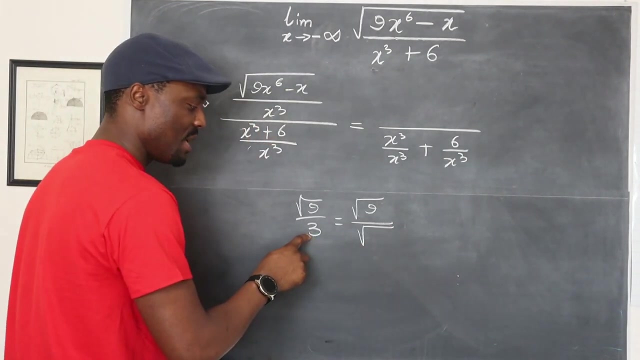 this number. So another way to do this is to write square root of 9 divided by 3 and then push this 3 under the square root side. It becomes square root of 9 divided by. write this as a square root, What will 3 be? 3 will be the square root of 9.. Ah, we can as well just write it as this. 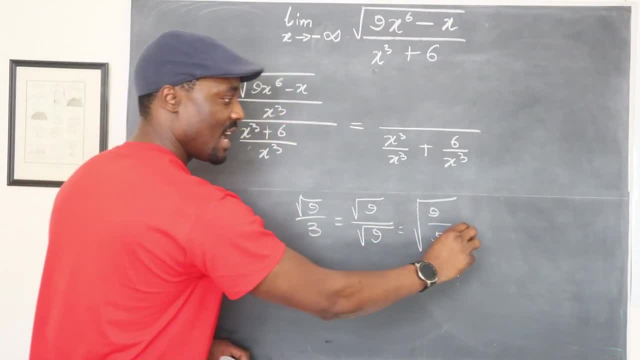 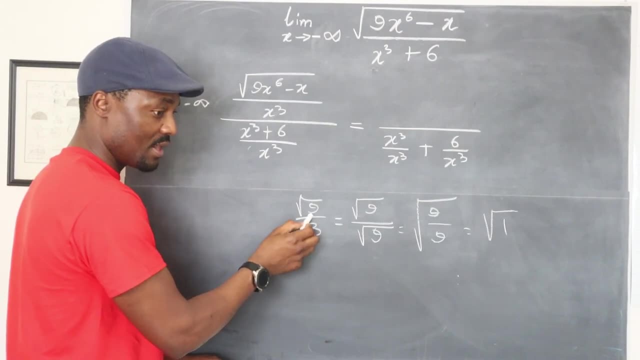 9 over 9.. Okay, this is allowed, and that gives you the square root of 1.. So you can see, for you to push a number under the square root side, you have to square that number and then it will stay under. So for: 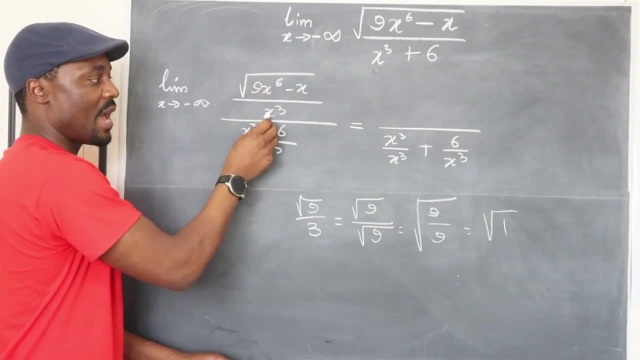 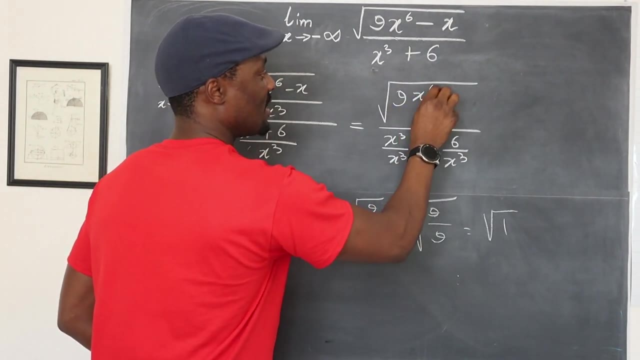 us to push this under the square root side. I have to square this, So x to the third will now become x to the sixth. So I can rewrite this as 9x to the sixth over x to the sixth minus, and then I can. 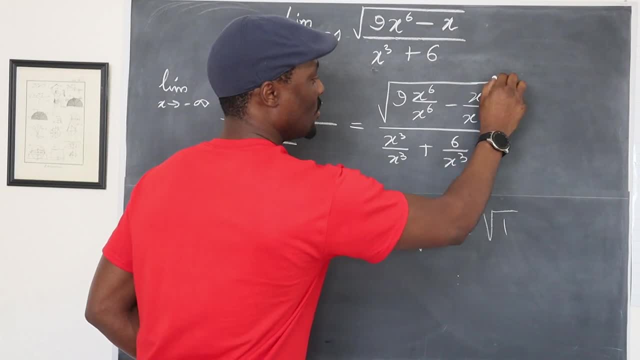 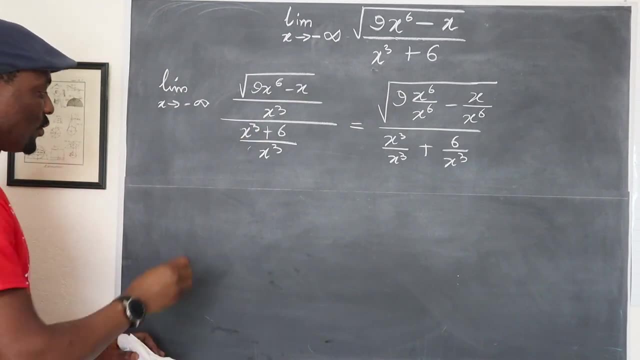 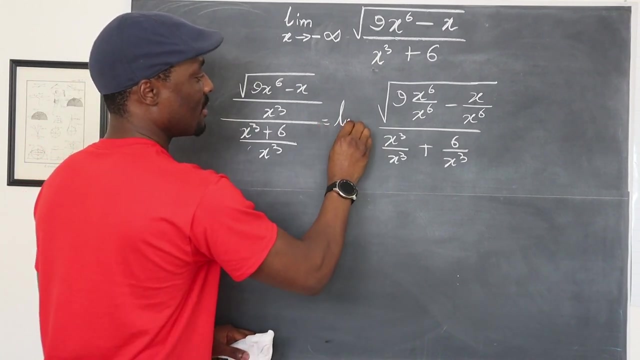 break this down also, x into x to the sixth. So this simplified our problem and we can get much simpler answers. So, oh, I forgot to write the limit sign. Well, don't ever forget that This will be equal to the limit of x as it approaches. 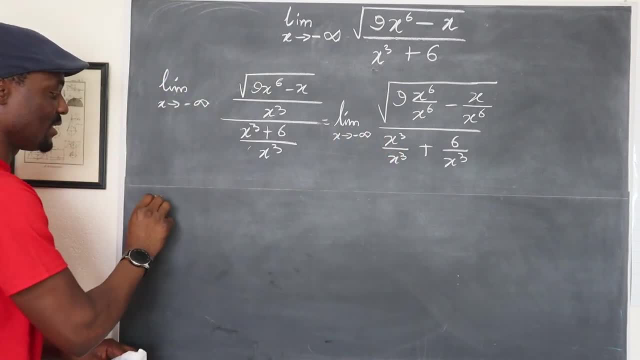 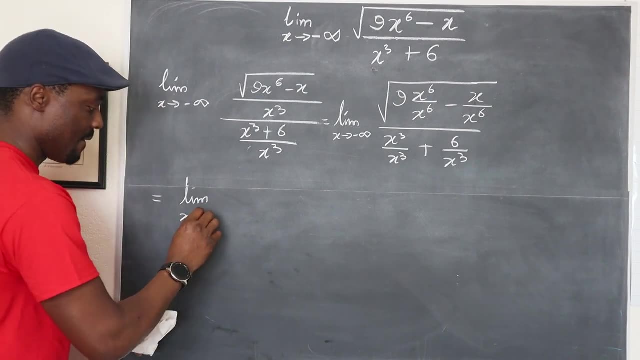 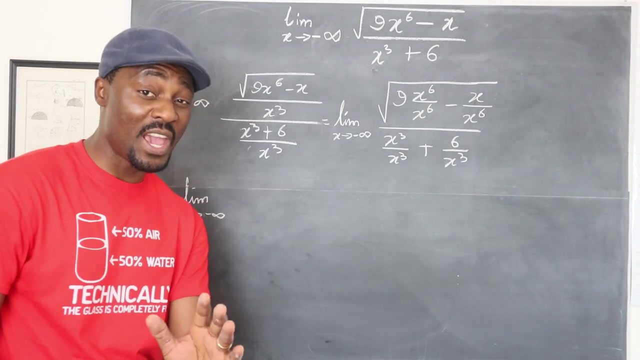 negative infinity. Don't forget to write that. So at this point it's going to be the limit of x as it approaches negative infinity. negative infinity of this is where you need to be super careful, You see, when you take the square root of anything. 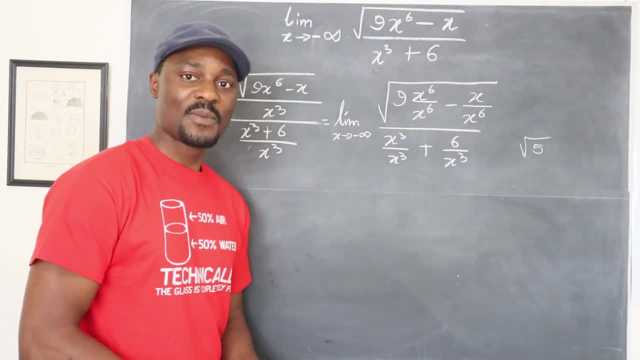 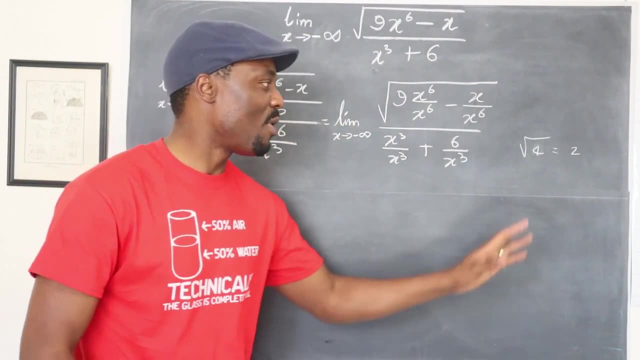 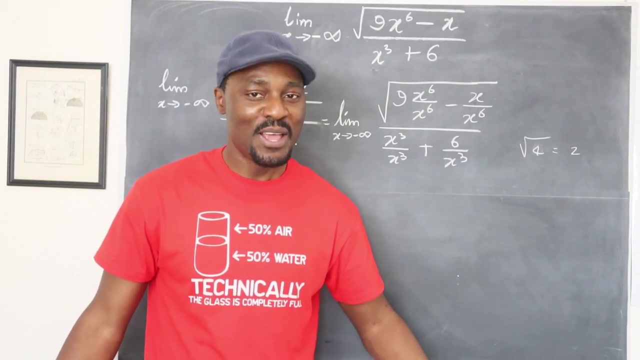 the square root of 5,. or let's take 4, the square root of 4,. there's a natural tendency to write 2, because most of the time the numbers would deal with positive numbers. natural numbers, okay, But this question specifically says that x is approaching. 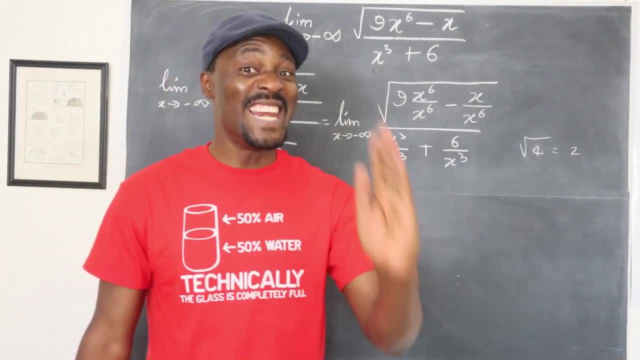 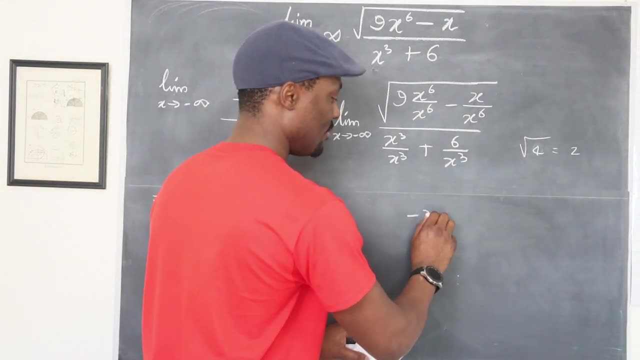 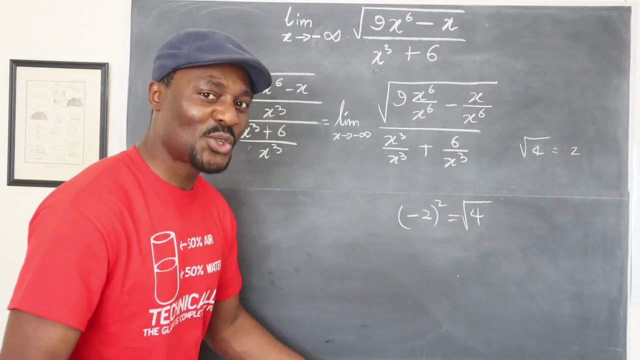 negative infinity, which gives you the impression that X is a negative number. okay, when you square it in negative number, like negative 2, and then you take the, you get 2, you get 4. when you now take the square root of 4, you're supposed to get negative 2, but naturally we don't remember that negative 2 is one. 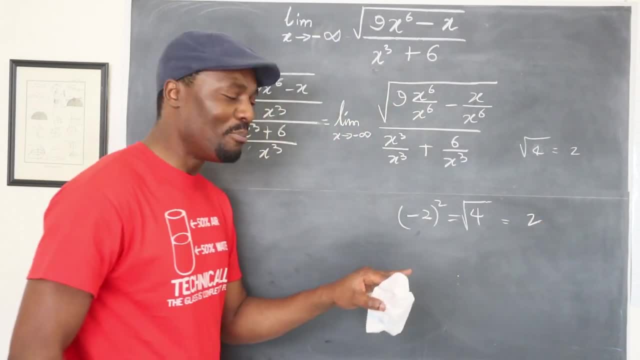 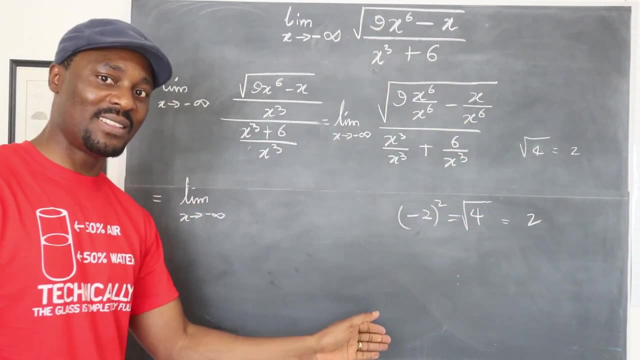 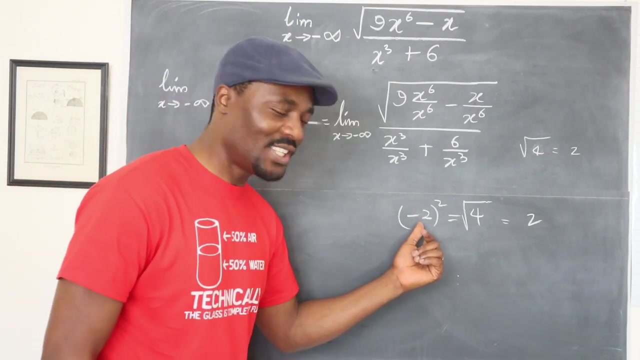 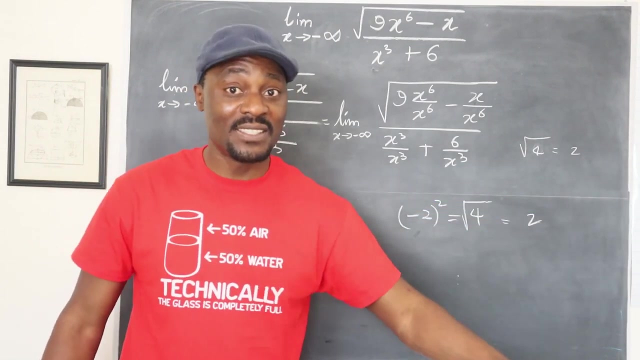 of the options. we just say the answer is 2, but we have changed it. so when you square negative infinity and take back the square root, what you've actually done is you're trying to take the negative sign away. don't do that. you have to recognize that X is approaching negative infinity, so X is a negative. 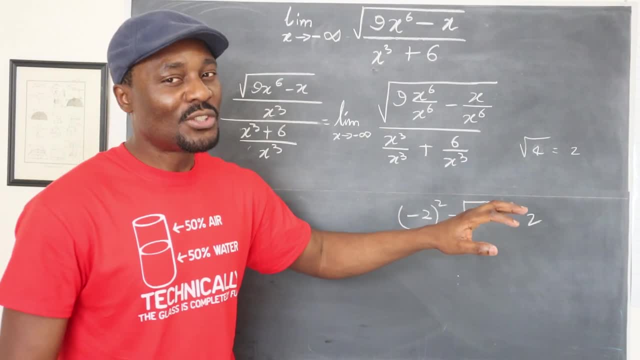 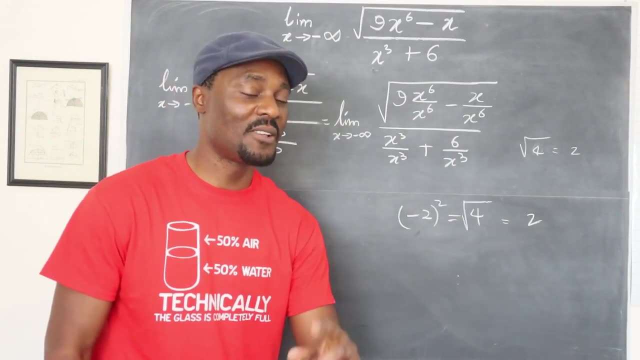 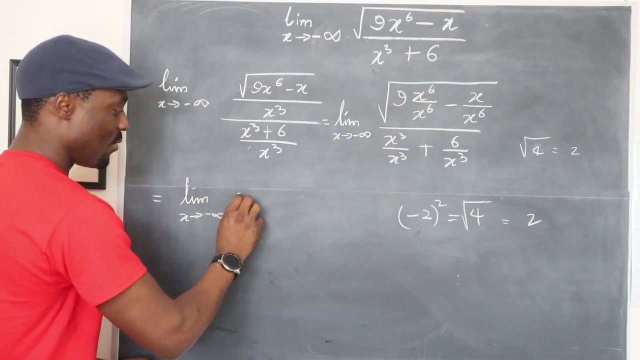 number. so when you take a square root here, just remember the negative sign. okay, it's gonna be a negative result. in order to not forget- this is the trick- just put a negative sign out there as soon as you cancel these out. so I'm gonna write negative. then what's left? these two will cancel out. I'll have 9. 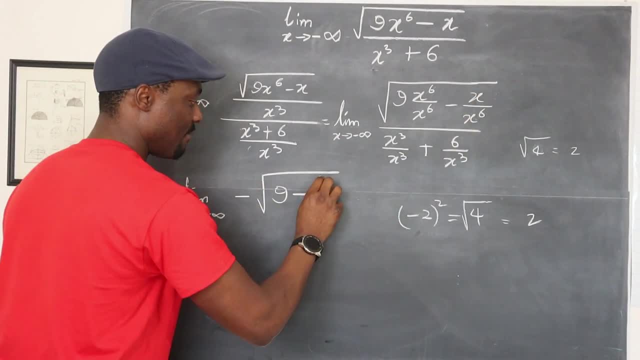 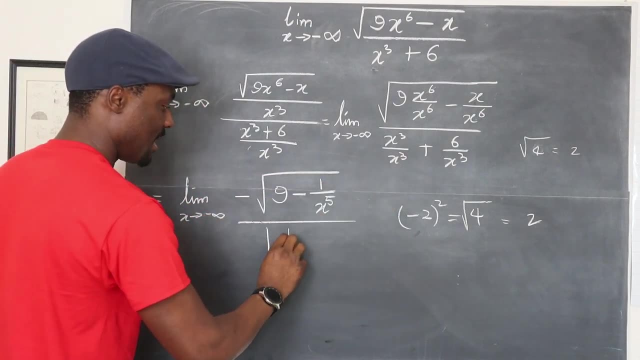 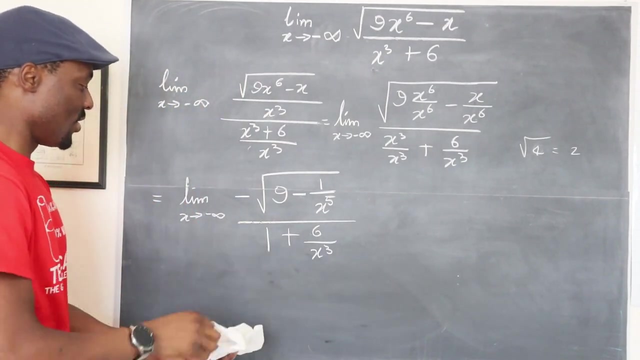 minus. this will take this out. if you have 1 over X to the 5th divided by- and then this takes this out- you have 1 plus and that's a 6 over X to the 3rd. we're almost done, okay. so at this point you. 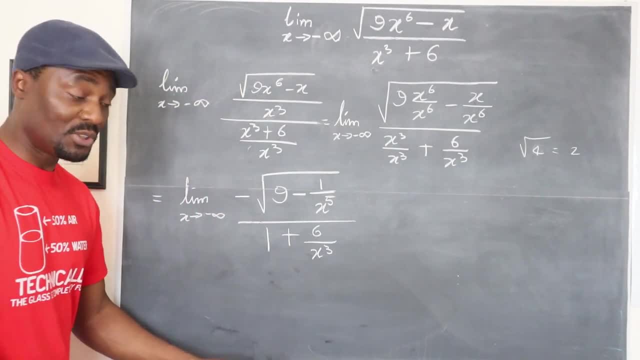 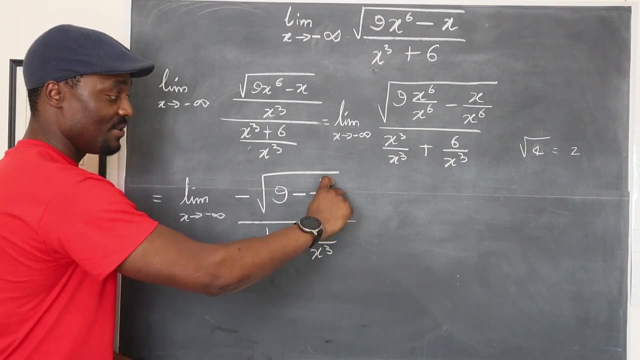 just need to substitute infinity in there. okay, some people will tell you you're putting negative infinity, so change the sign to positive. it doesn't make any difference, because you're gonna keep on. this is gonna give you 0, this is gonna be 0. remember, if you divide anything by infinity, your answer is 0. so 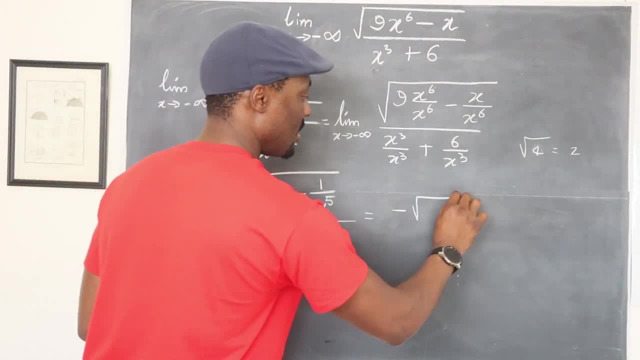 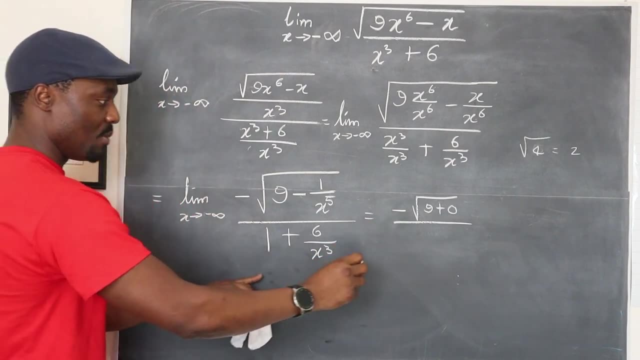 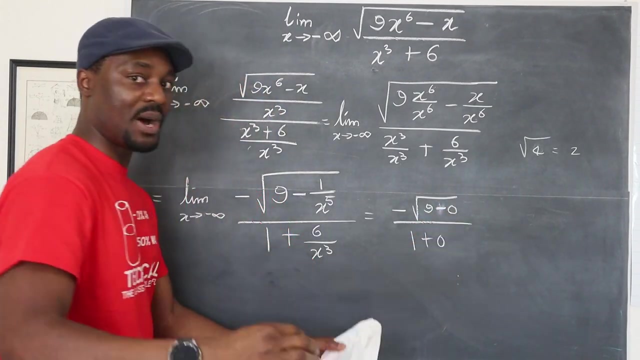 put infinity here, you're gonna end up with negative square root of 9 plus 0 or 9 minus 0, whichever you choose. okay, and then this will be 1 plus this is gonna be 0. okay, I just want to leave this as negative. okay, since this is 0, there's no. 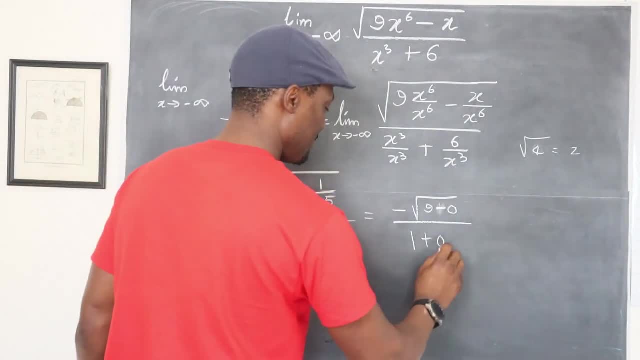 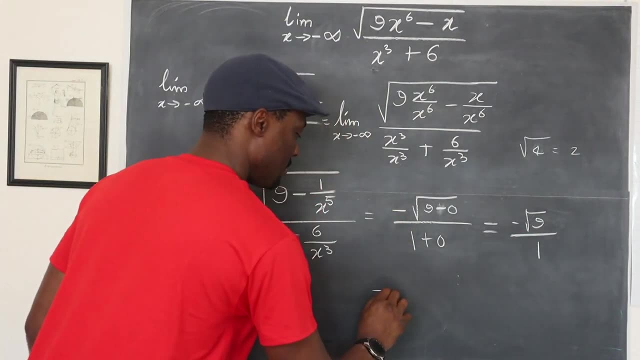 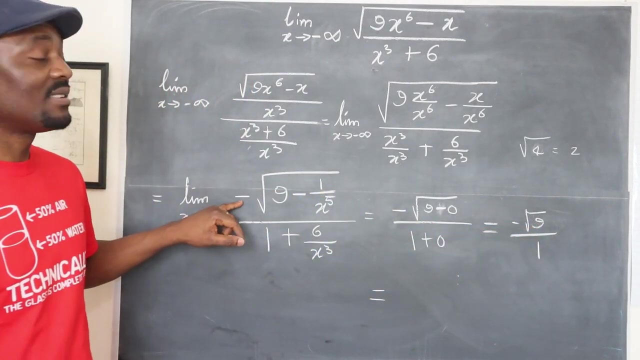 positive or negative, 0, so it's the same thing. so you end up with negative square root of 9 over 1. so see, now you don't have to be reminded that the number is negative because we already put the negative sign here. so that's all you have to do. what's the square root of 9.. it's 3, so it's negative.